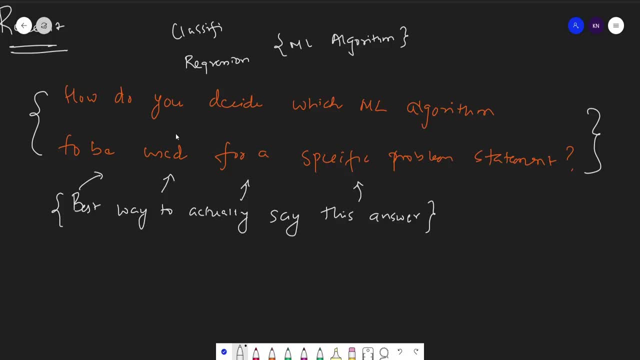 interviews, you know many people come up with this particular question: how do you decide which ML algorithm to use for a specific problem and how do you decide which ML algorithm to use for a specific problem statement? okay, and I've seen many people giving different different answers, various different answer. okay, but what is the feasible way that we 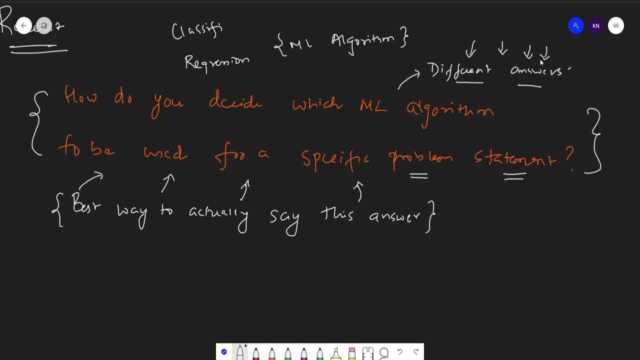 should basically tell in the interview: please write down your comment. write down your comment in the comment section of this particular video and, before I give you the hint, you know what do I feel or what should be the hint that is to be given to you in order to answer this. it is pretty much simple, guys. 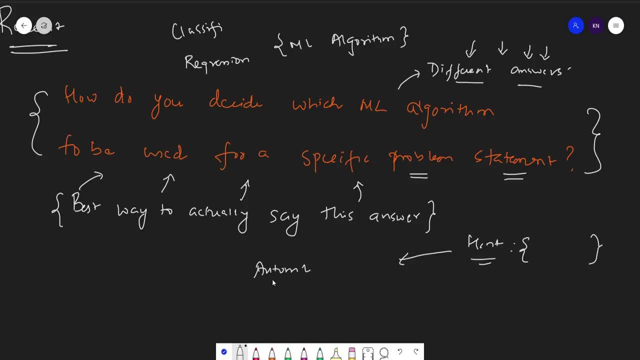 think of a auto-ml solution. okay, how does the auto-ml work? okay, take any auto-ml example. okay. auto-ml basically means you take Pi caret, you take H2O, right, H2Oai any auto Evidence, any auto-ml solutions. okay, and just think: how do this solve a? 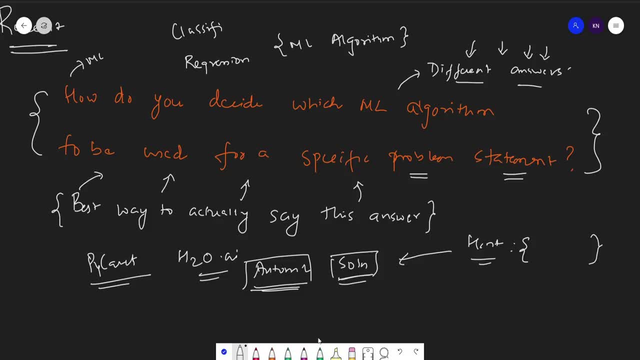 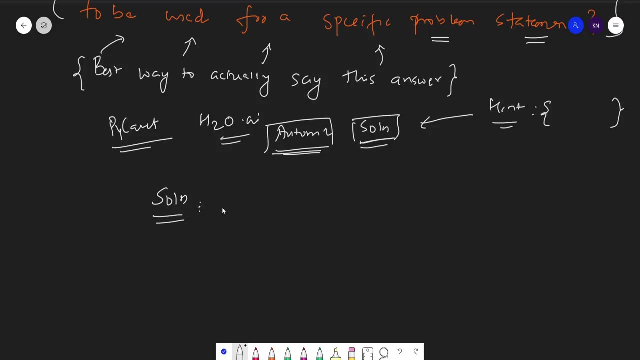 specific ML algorithm. sorry, a specific use case. you know a specific use case case. how do you, how do they solve this specific use case? you know guys for this? if I think of a solution, the best way to answer this in an interview is that try to apply. try to apply every algorithm, okay and based on the performance matrix. 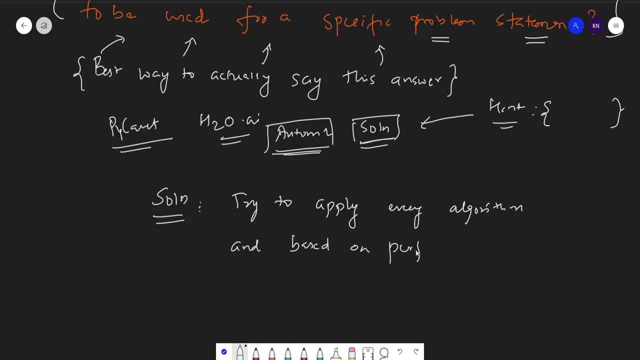 based on performance matrix. okay, try to select the best algorithm, okay. so what? I feel this is the exact. this is a proper solution to basically answer this particular question, because if you say okay, if there may be also different people like who will be saying, if the data set is not linearly separable, then 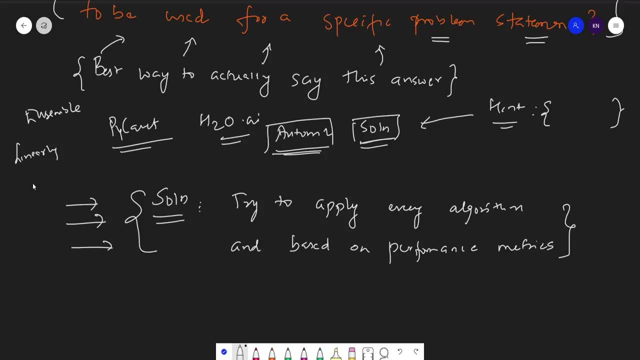 I may go with ensemble techniques. okay, if it is not linearly. if the data is linearly separable, okay, I may go with logistics regulation. I may go with naive bias. if the data is having text data, you know I may go with this technique. okay, over here, you know. 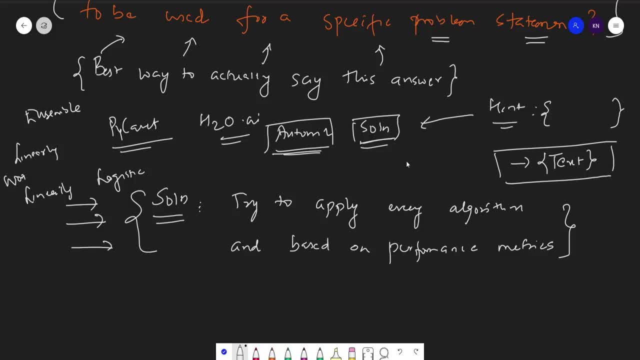 they may ask you some more additional question which, again, you will get confused in the later stage. okay, so that is the reason why I am saying you that always try to follow this particular approach, to say that how to apply every we we really need to apply every. 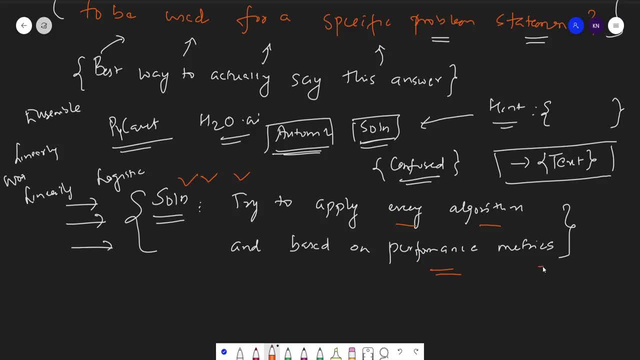 algorithm for a particular problem statement and based on the performance matrix. why i'm also taking performance matrix? because based on other other domain, you know, suppose i'm doing some medical health data. okay, um suppose i want to predict whether the person is having diabetes or not. so in this particular case, i need to really think on the performance matrix. what should we? 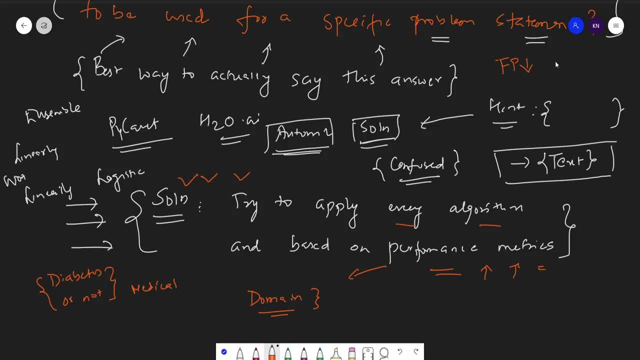 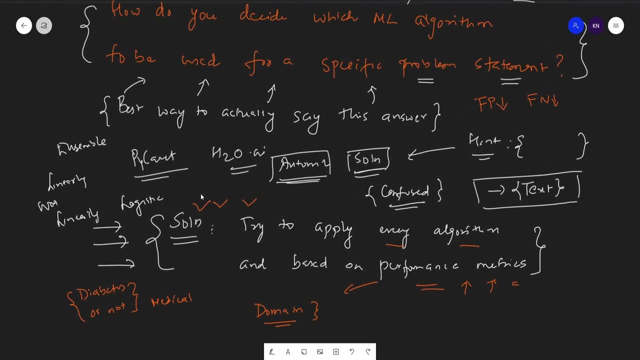 focus on reducing, whether we should be focused on reducing the false positive or false negative, or both. based on this, we'll decide the performance matrix, where we have different, different performance matrix. why i'm making this video? because recently- um, you know this- was asked to one of my subscriber again. he told: uh, these all things if our data set is not linearly separable. 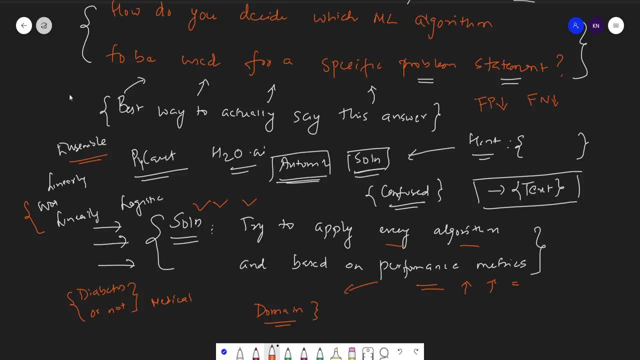 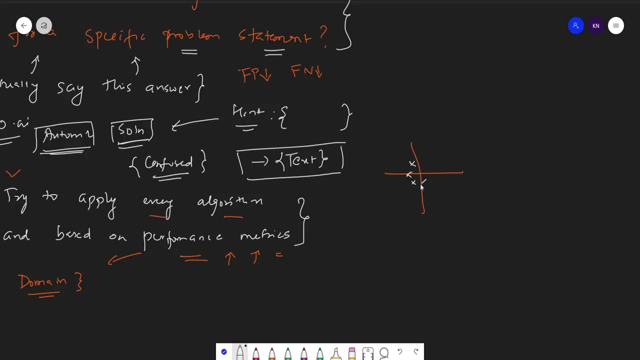 we may basically use ensemble techniques. then they started getting more and more questions. they just said that in logistic, don't you think we'll be able to solve with non-linear, separable data. then that person said no. then they gave them his him a specific example where they told: is that suppose, what if my data points are something like this? 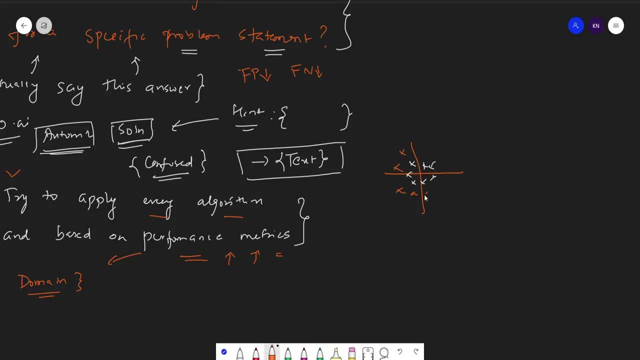 you know, suppose my data points are something like this, will i not be able to use a linear regression- oh sorry, logistic regression to classify this particular point? right? so there was technique. we basically have to. there are techniques how we can actually solve this non-linear, separable data. so i'm telling you, in order to get prevented from this kind of questions: 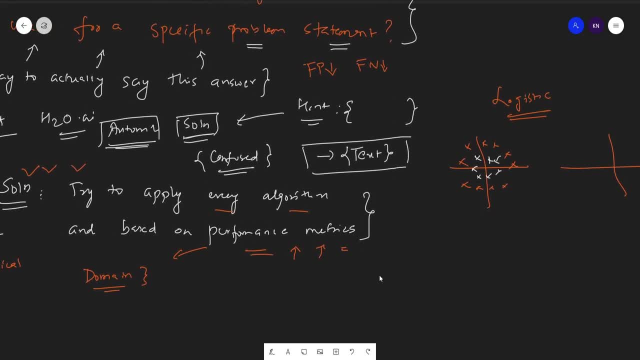 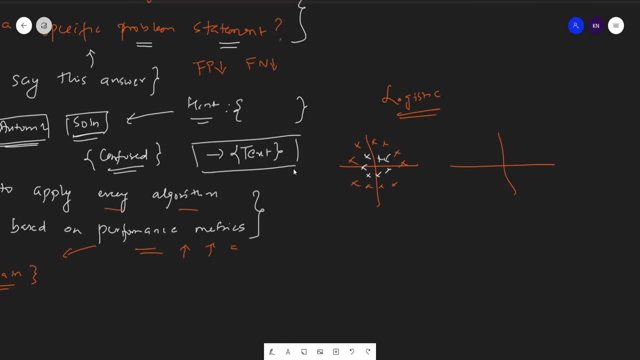 you know, in order to make your, we have a proper way to basically convert this data by squaring this feature. suppose, iır, suppose, if i square this x2 and y2, then i may be getting this information something like this: properly splitted, properly split, and you, you?